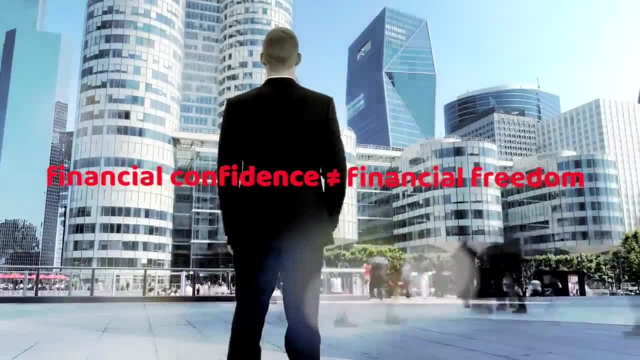 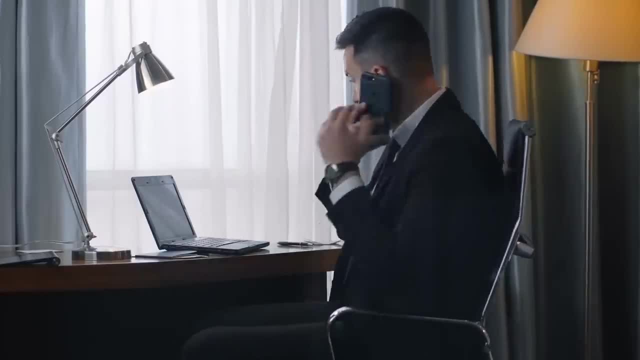 financial confidence. It is different from financial freedom. This is because freedom is based on the amount of money that you have available, while financial confidence is based on your confidence and acumen to generate money. Now, here's the thing: most people think that. 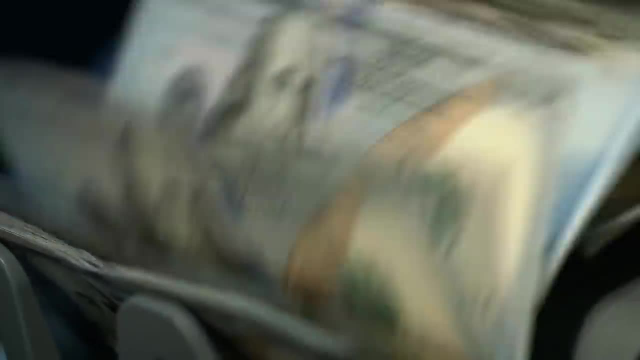 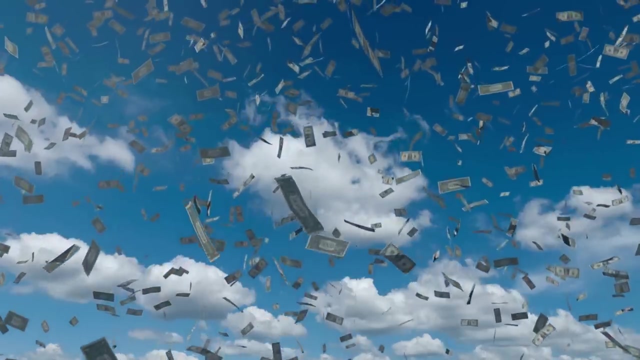 there is a money scarcity. Most people think that there is a money scarcity. They think that there is no money and making more money is impossible, But this is deeply untrue. The truth is, the world is littered with money, but only those with the skills and knowledge. 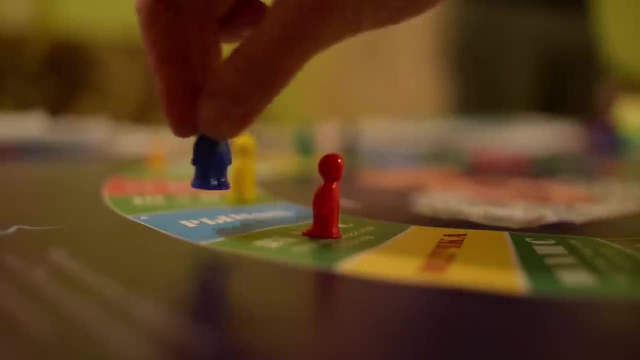 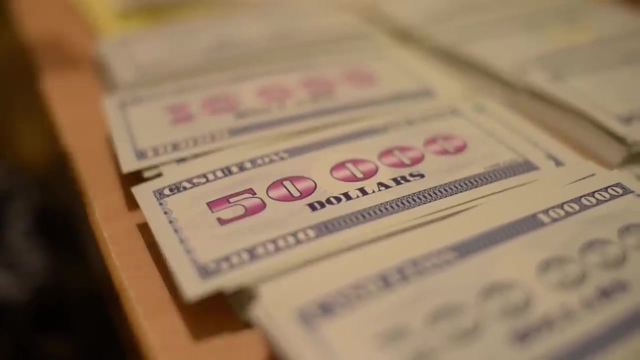 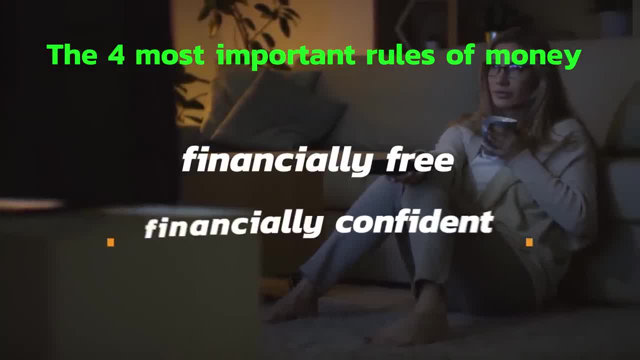 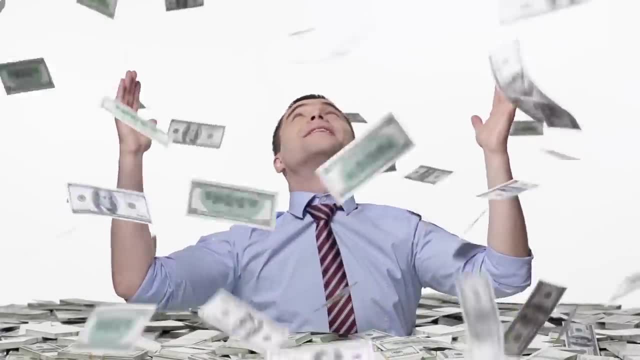 the basics of being financially free, financially confident and financially literate. These simple rules that I will give you today will elevate your money game and take you to a whole other level you've never seen before, as long as you are hungry and dedicated. 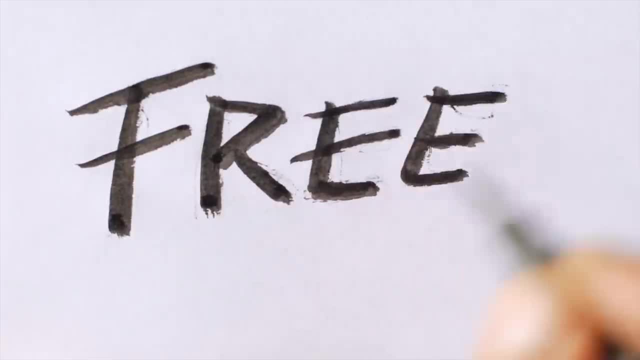 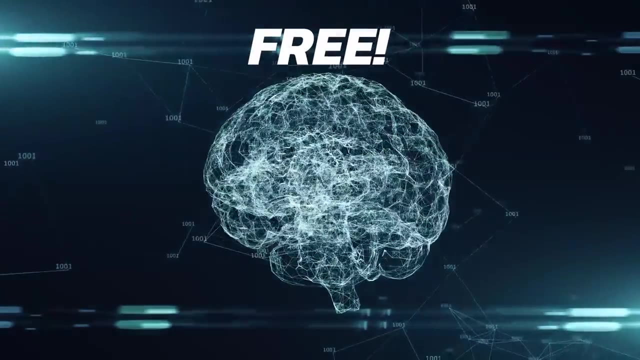 I'm going to give you all of this information for free. I don't sell books, webinars or online courses. All the knowledge on this channel is free. so if you want to show your appreciation, click that like button and the subscribe button right now. 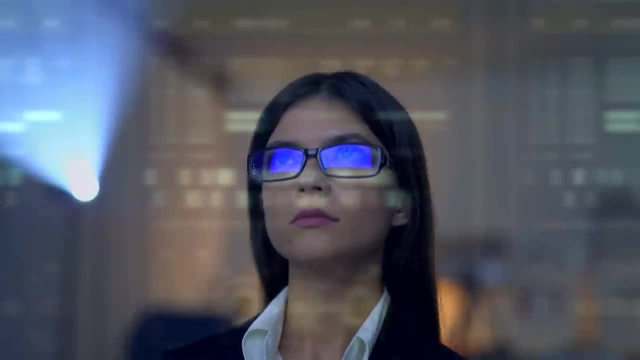 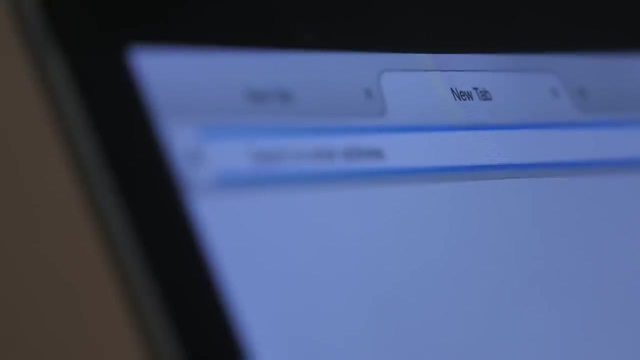 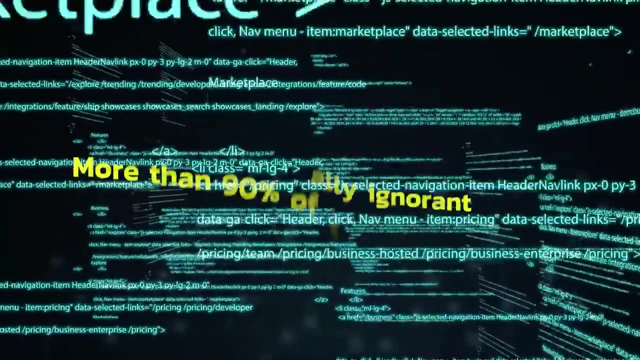 It is actually very fascinating how all this information is becoming more and more available every day for very cheap or even for free, And everything is easily accessible with a couple of Google searches. So even if everything is at their fingertips, more than 90% of the population is still financially ignorant. Let me give you a quick example. 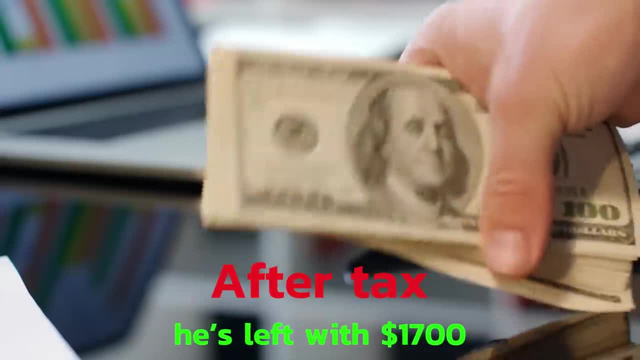 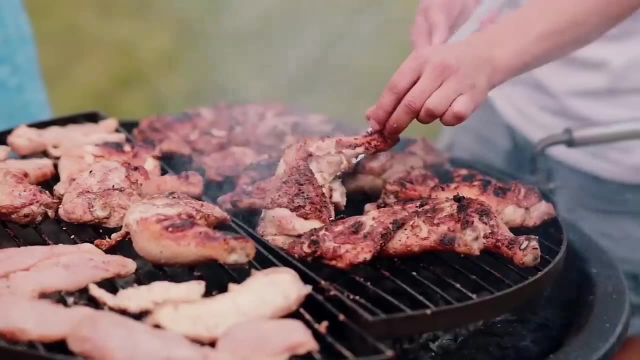 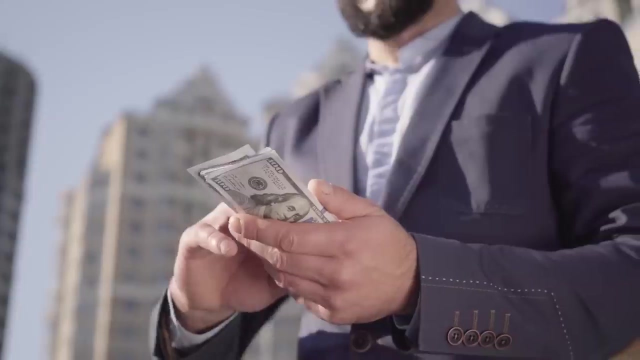 Peter just got his monthly paycheck. After tax, he's left with $1,700.. Instead of using this money to invest, save or anything else that might be useful, he decides to waste it on a couple of barbecues with friends and many other useless liabilities. Are you a Peter? Because there are. 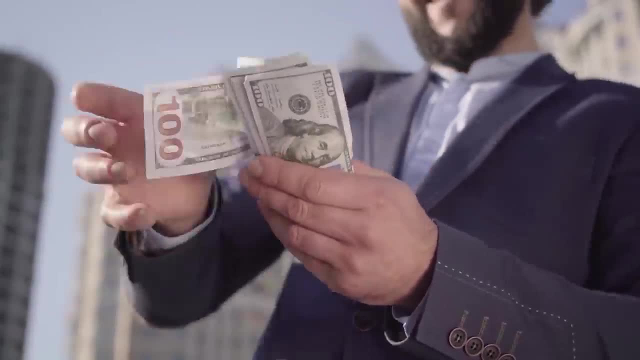 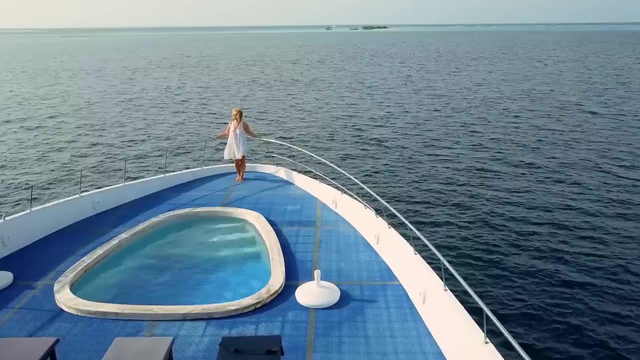 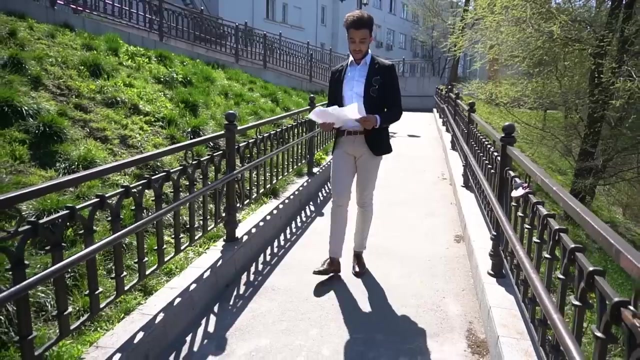 unfortunately, a lot of financially ignorant people today. but the thing is, if they can change a few bad habits and develop a rich mindset, just about anyone can become rich. There are no rich people that are financially ignorant, Except of course for those that got lucky, For example, stumbling 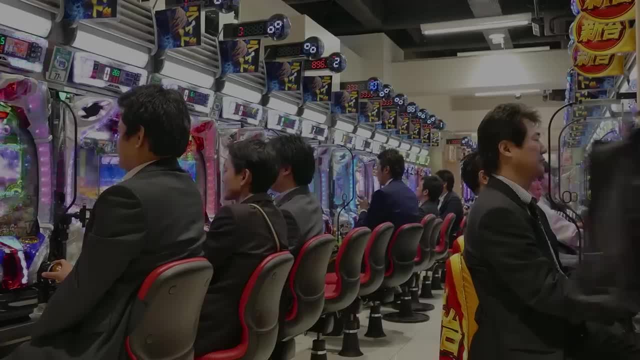 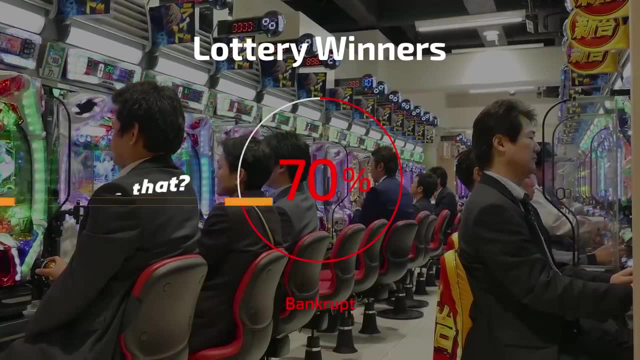 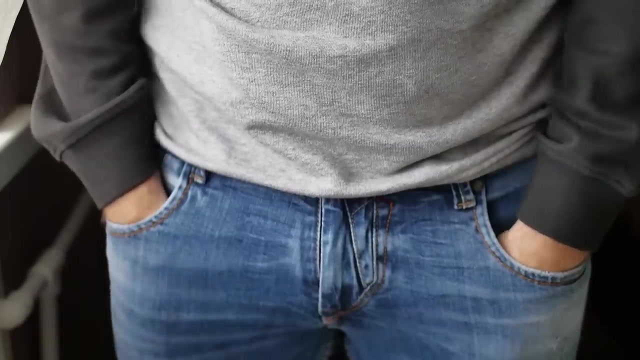 upon a large inheritance or winning the lottery. However, statistics show that 70% of lottery winners end up bankrupt after just a few years of being extremely rich. Why is that? Again, it all comes down to how financially educated one is. If you have a lot of money, you will still make bad decisions and lose it all because you don't know what to do with it. So if you want to become rich long-term, you need to have a lot of money. If you have a lot of money, you need to have a lot of money. If you want to be rich long-term and not just for a couple of years. 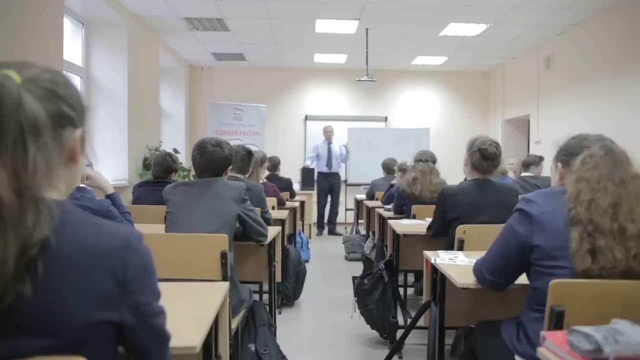 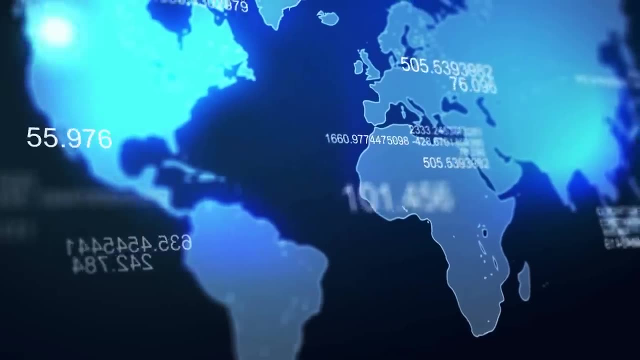 you have to get financially educated. Unfortunately, this kind of education is not taught in schools, so you need to do it by yourself. So all the information is easily accessible, and this raises the question: why don't people learn more about finance? 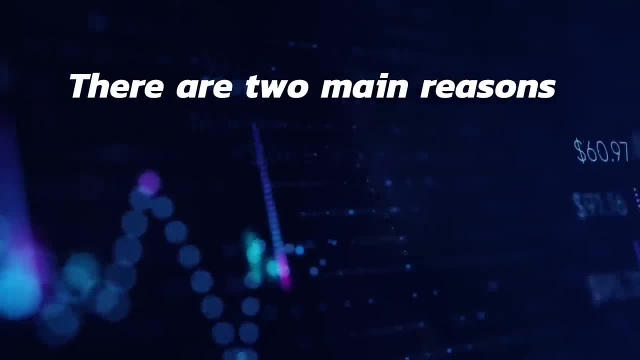 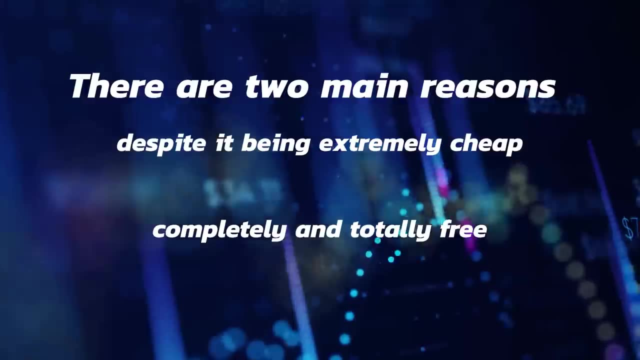 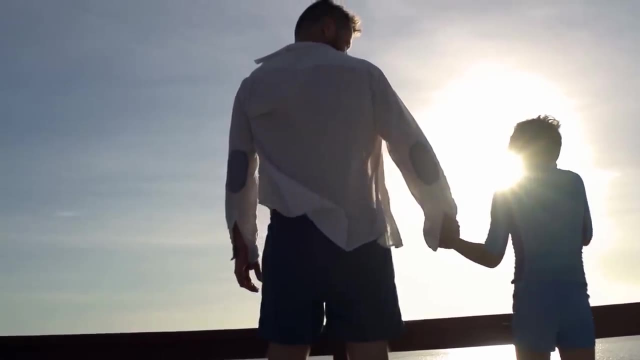 There are two main reasons why people don't get the financial education they need, despite it being extremely cheap and, in some cases, completely and totally free. Reason number one: conventional wisdom. Here's the truth. financial education is not conventionally okay. Most people will give you a mindset of scarcity, and if your mindset is, 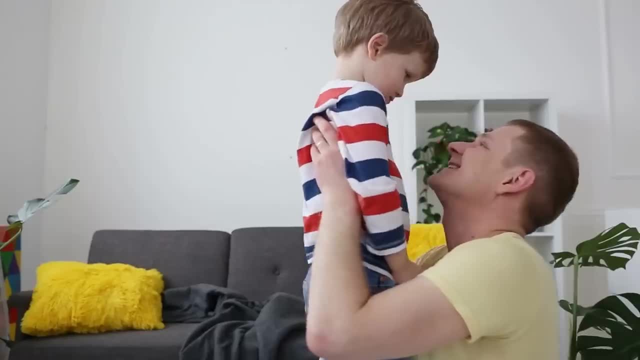 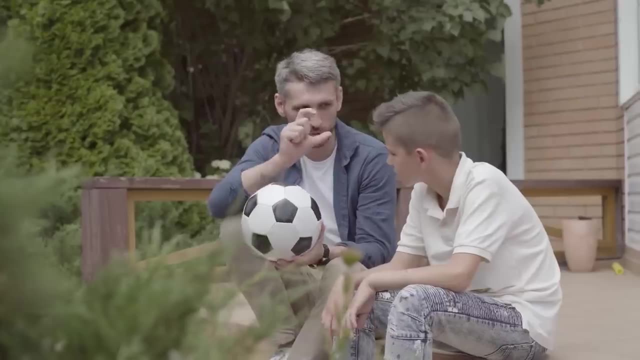 wrong, you will never attract money. For example, growing up your parents might have been telling you money doesn't grow on trees and money is the root of all evil. These lies that people tell their kids are stopping people from taking the necessary steps to a better life financially. 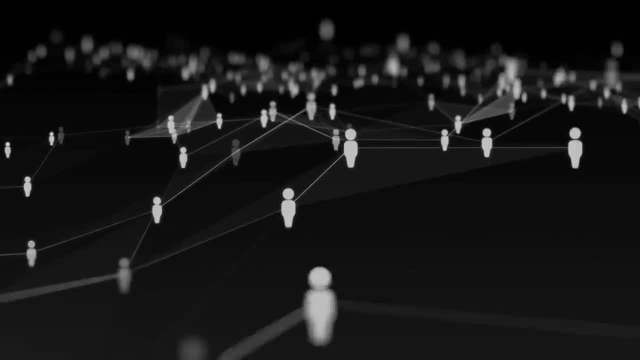 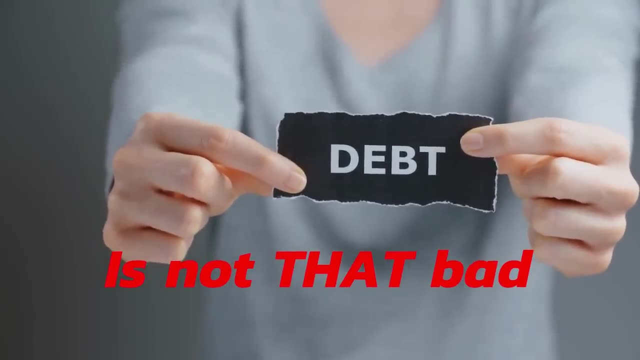 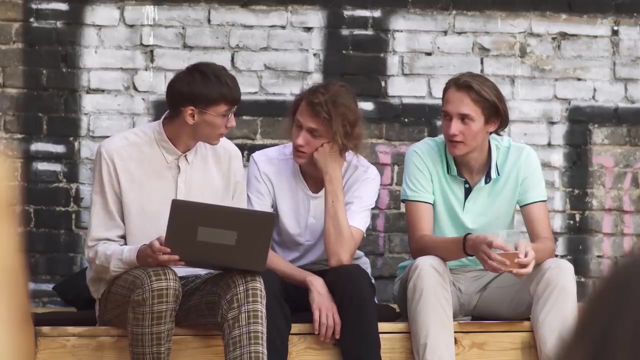 Another conventional concept that is widely thought but is extremely wrong is the negative connotation towards debt. Debt is not that bad if you know how to use it, but still people demonize it because they don't have the appropriate education. So you have to stop listening to those that aren't financially literate and financially 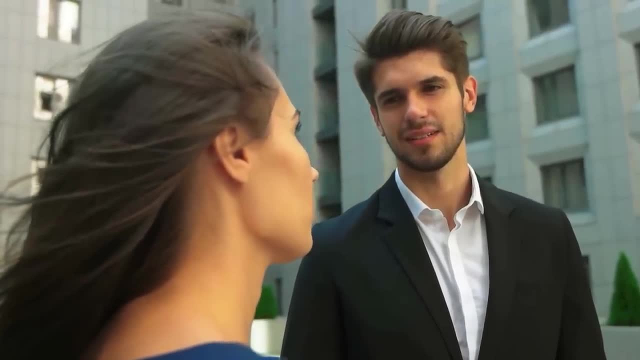 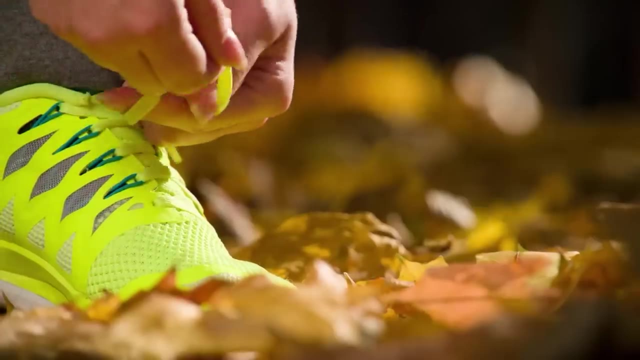 confident. You should start listening to those that actually know how to generate money, because they are the ones that can give you tips on how to become financially educated. Just like in a sport, you can't just learn it from someone who has never skied before. You don't want to learn how to ski. 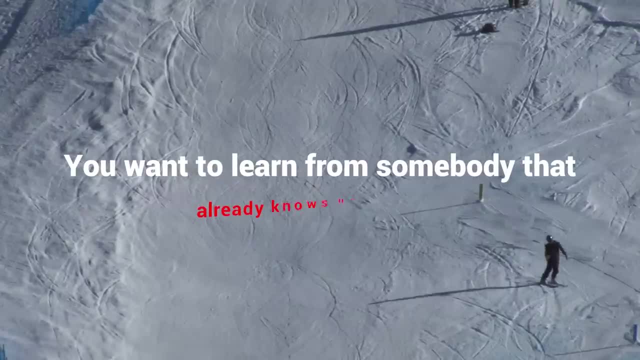 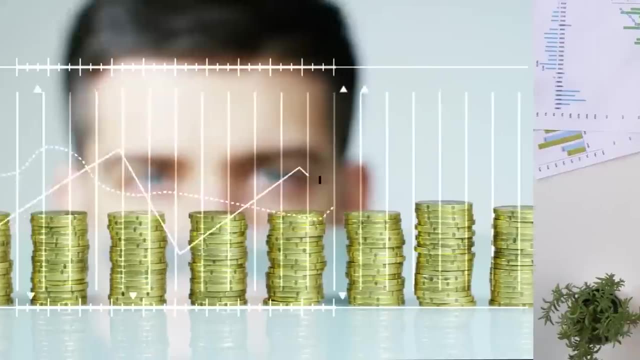 from someone that has never skied before. You want to learn from somebody that already knows how to do it. Apply this to your financial education and you'll learn very fast. Reason number two: comfort zone and self-esteem In order to generate money. 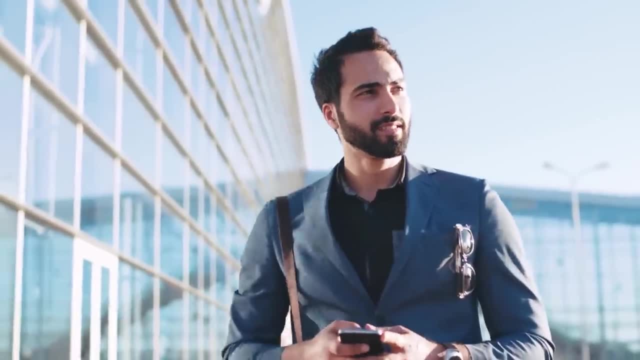 it's believed among the rich that you need to be confident and have decent self-esteem. Self-image is important and you have to first of all believe that you truly deserve to be wealthier and happier. If you don't, you're just being a fool. If you don't, you're just being a fool. 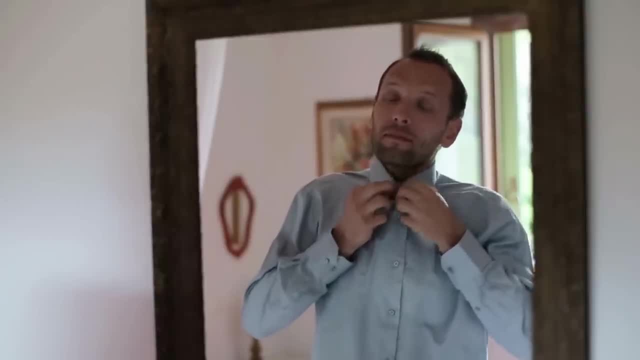 There are so many reasons for this, but the reason I'm talking about is that if you don't, you're just being a fool. If you don't, you will never become rich. Think of it like a self-fulfilling prophecy. you have to see yourself rich first. 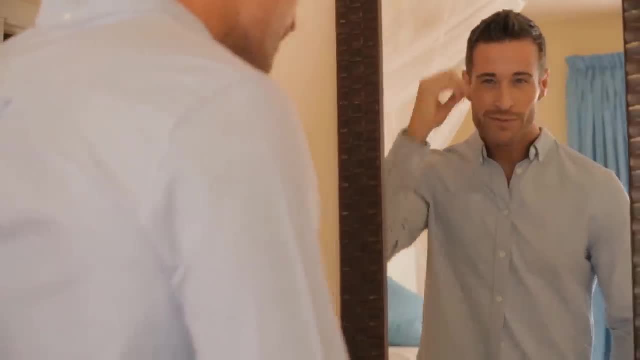 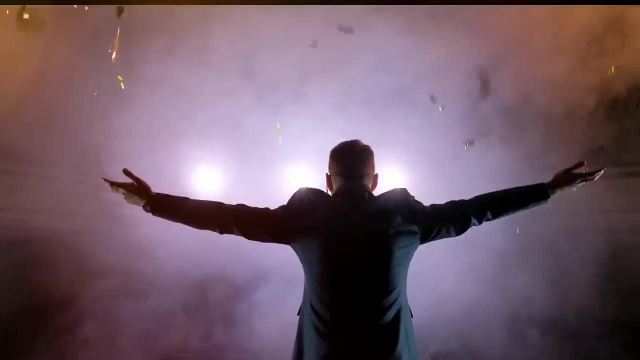 This confident, charismatic, rich image you see yourself in your mind will give you the needed confidence to continually act out of your comfort zone, which is very important. A very successful person once said: most people are not successful because they are afraid of success. 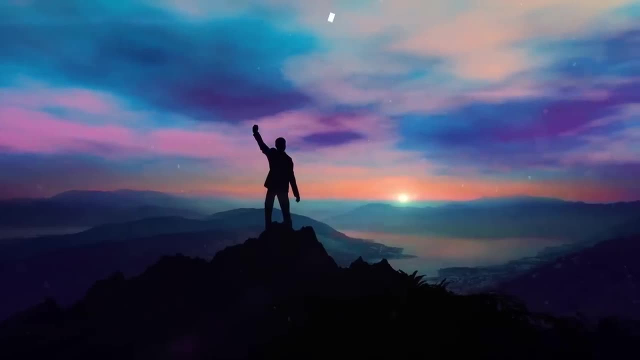 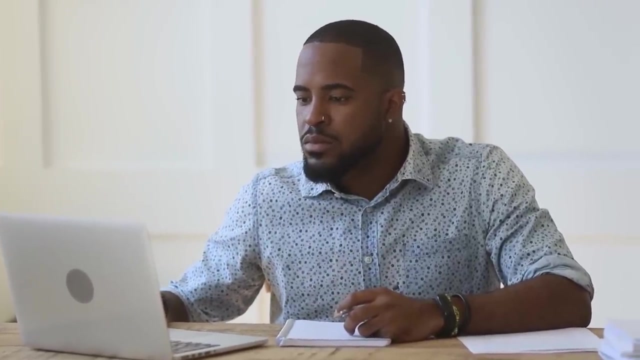 This is true. In order to become successful, you have to step out of your comfort zone and take risks. For example, if you want to start your first business but you don't have any money, you might first of all have to take the risk of getting a loan from your bank and putting 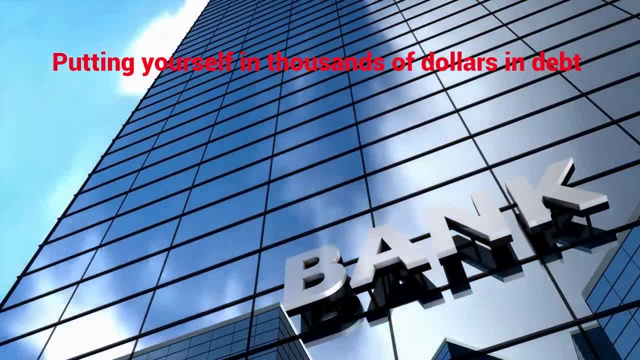 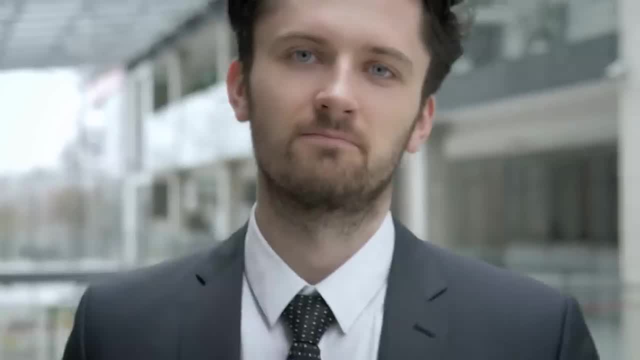 yourself in thousands of dollars in debt, which is out of a lot of people's comfort zone. Charisma and confidence are some of the key ingredients you need to become rich. If you don't have the confidence to take action, you will never become rich. 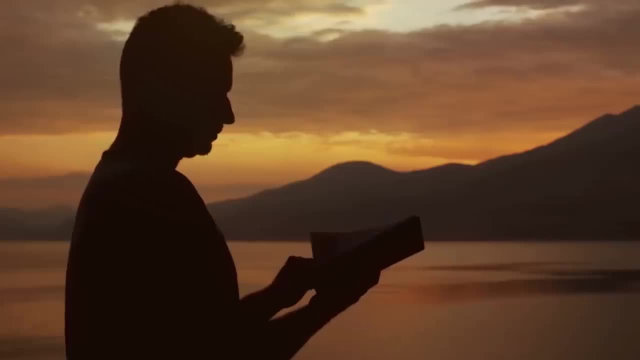 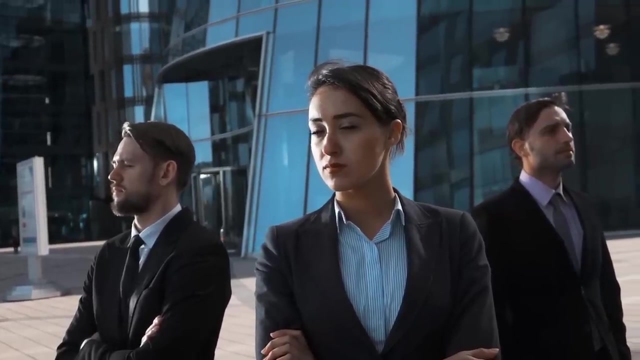 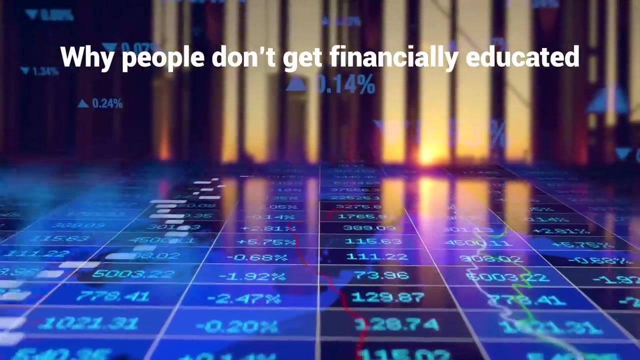 So before actually getting into financial education, You have to first work on yourself and your mind when it comes to risk taking and failure. Confidence will give you the strength and the courage to take risks and perform under pressure. So now that you know all about why people don't get financially educated and the importance 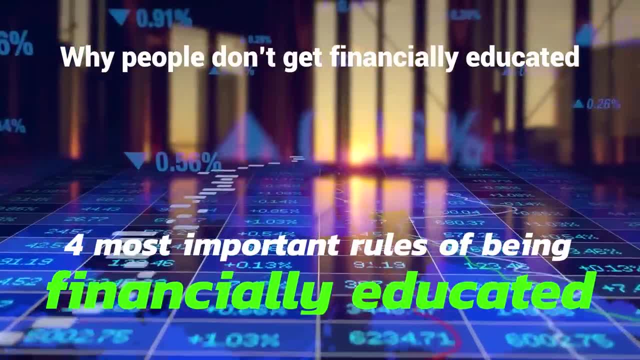 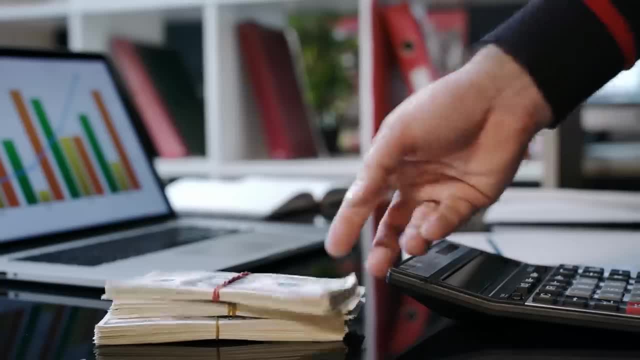 of it. let's get started with the 4 most important rules of being financially educated. Rule number 1,: don't invest in what you don't understand. Investing is very important, especially when you want to multiply your money. Here's the thing. 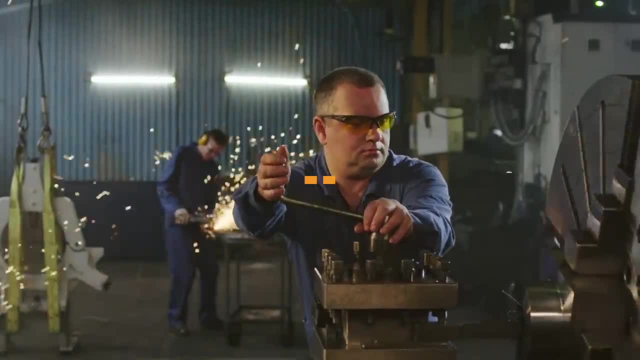 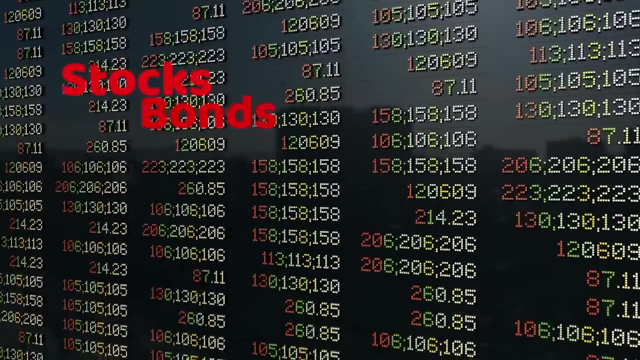 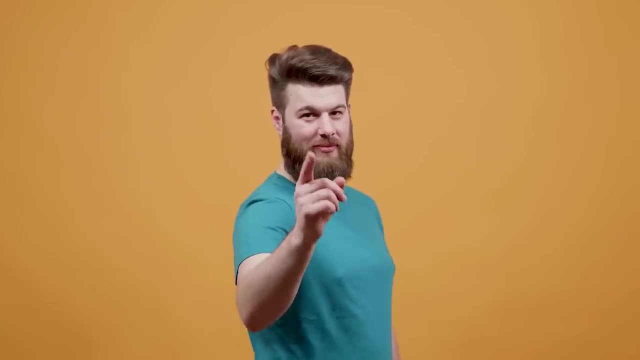 You will never, ever get rich long term by working for someone else. You have to start investing. There are many types of investments, such as stocks, bonds, real estate and forex, just to mention a few, But I want you to know the single most important investment, and that's in yourself. 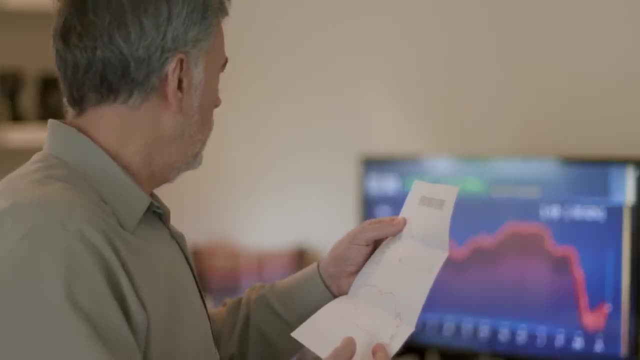 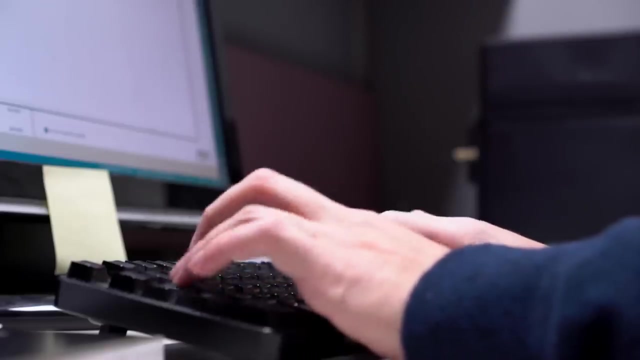 Invest in yourself Before investing in anything else. you have to invest in the development of your money making machine, your brain, getting the knowledge necessary to operate a business. operate a business, financial education included, is not optional. Your industry and your niche are. 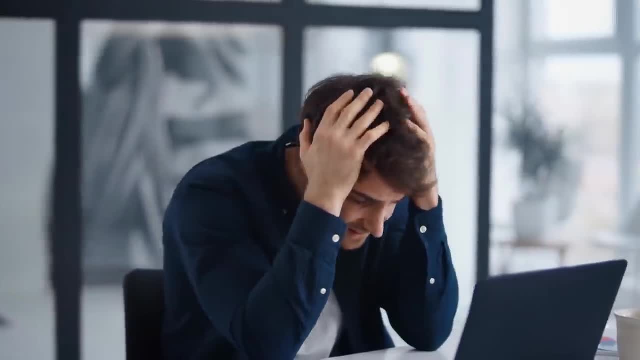 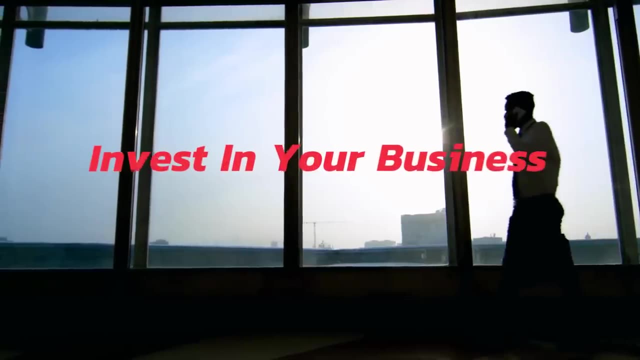 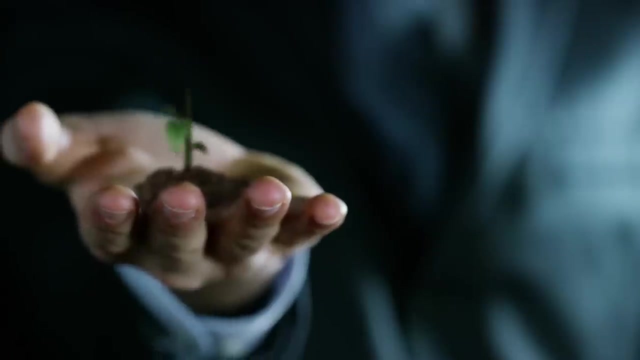 going to eat you alive unless you are always updated on what's going on. Stay up to date on all information that matters to you and to your success. Invest in your business. If you buy or create a business, you will probably, at one point, want to expand it. If you want to do so, you need 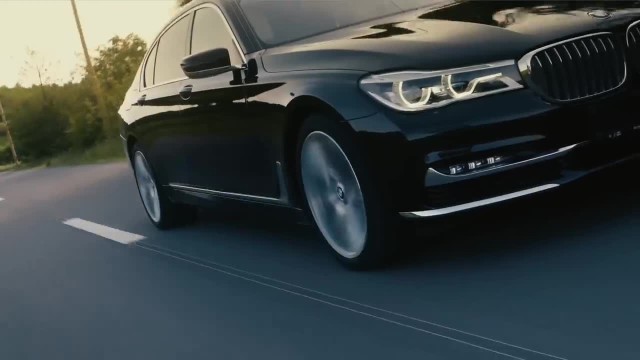 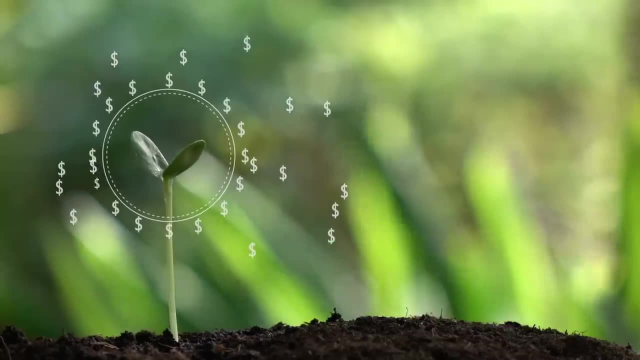 to put some money into your business in order for it to grow. It's like a car: in order to make it run, you have to put gas in it, And a business is no different: In order to keep growing, it needs to be fed money. Investing in your business might be anything from marketing to research or 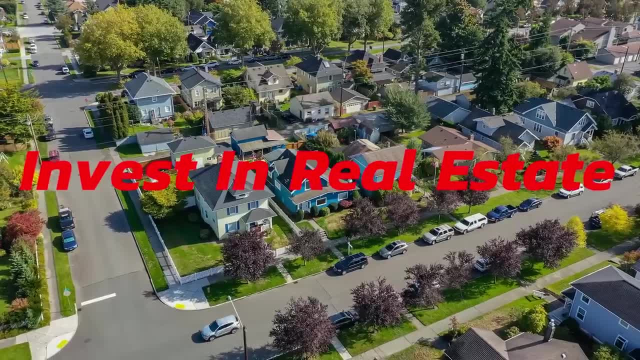 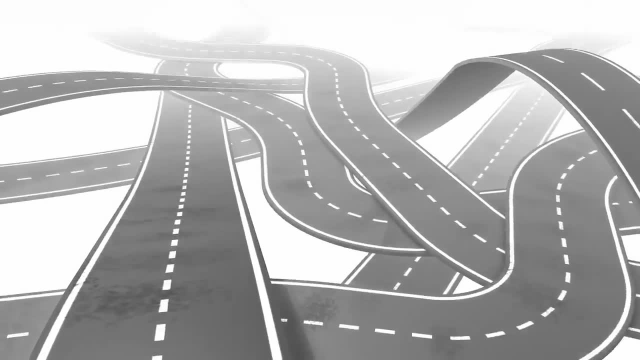 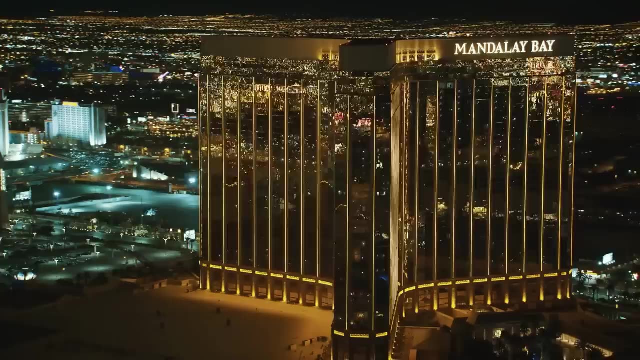 developing a new product. Invest in real estate. Real estate investing, like other investments, are basically buy low and sell high. A simple concept with very complicated steps. Most real estate investors start with regular homes, then they move to commercial real estate hotels. 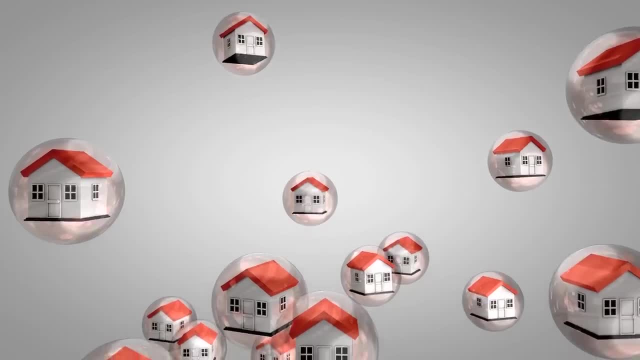 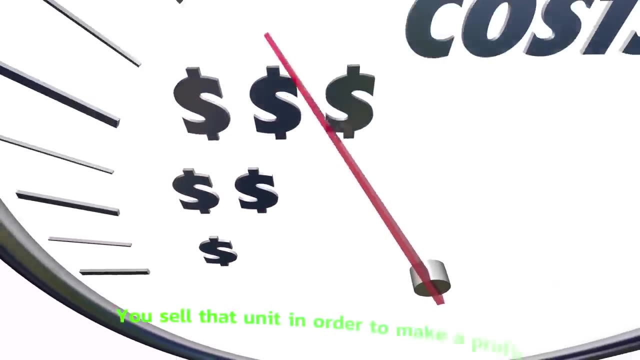 big commercial homes and then they move to commercial real estate. You find units, structures, with potential that have been mistreated. You fix them up, you wait for the price to rise and then you sell that unit in order to make a profit. 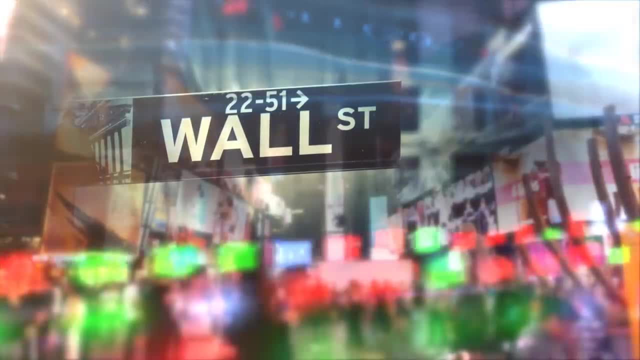 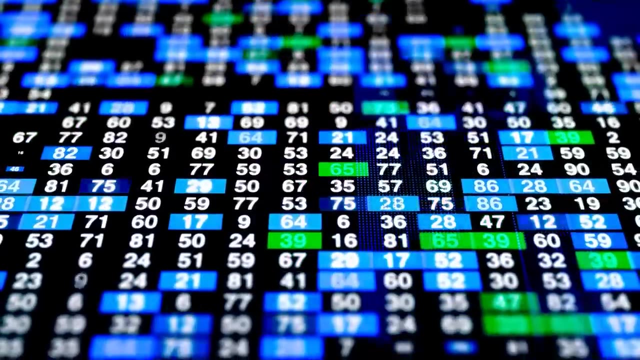 Invest in stocks. Stocks or shares are literally part of a company that is for sale to the public. When buying stocks, you have the right to a part of the profits of that business, which is the equivalent of your initial investment, Just like any other investment. 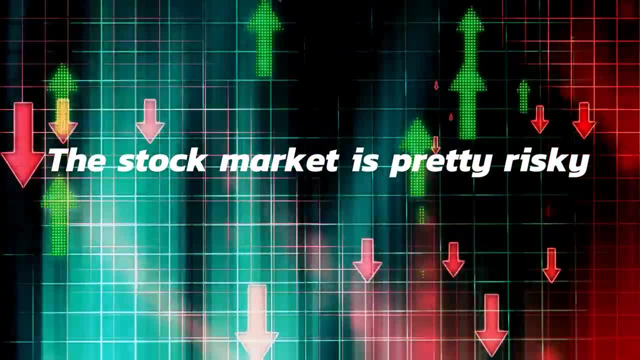 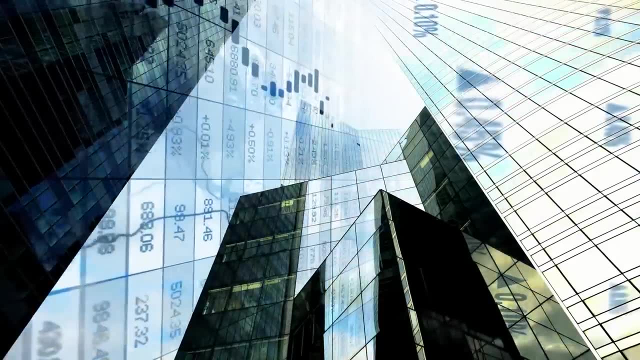 the stock market is pretty risky and there are a lot of people that lose a lot of money with it. So these four are the most important and well-known types of investments. However, independently of the type of investment that you choose, you have to know what you're getting into. There are rules to follow, but equally 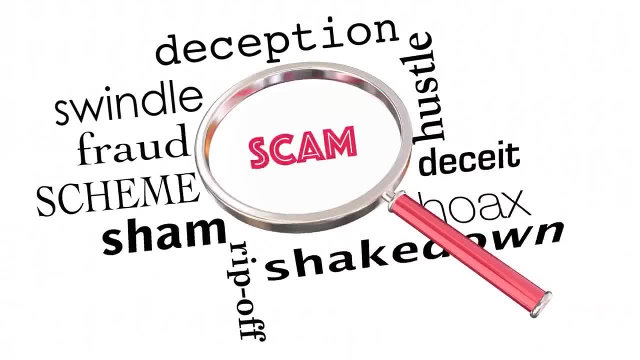 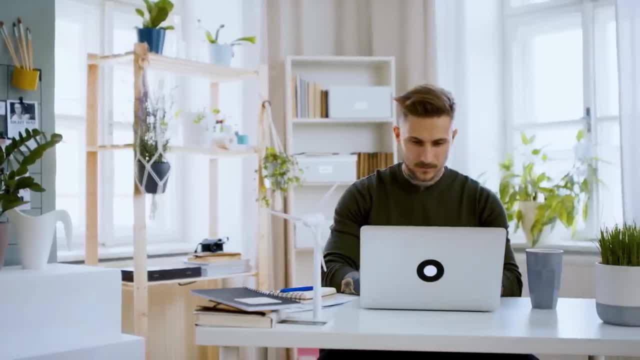 there's a lot of misleading information out there. A lot of people are willing to scam you just to take your money. So you have to be very, very careful who you listen to. do heavy research before putting your money in something new, or seek advice from a professional. 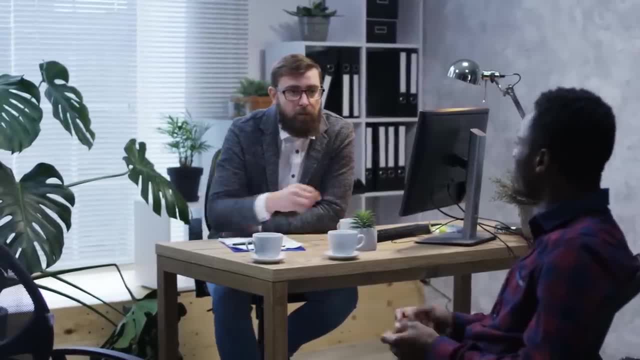 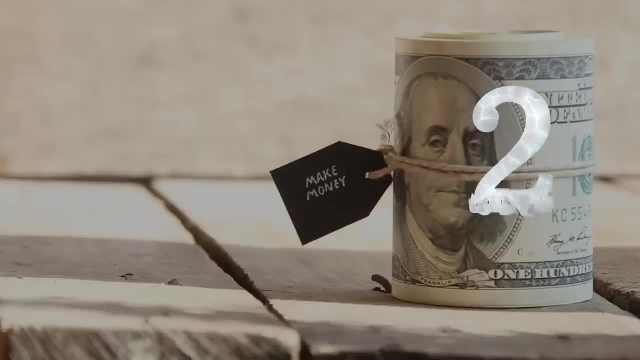 in that industry, You have to be very, very careful who you listen to or seek advice from a professional in that industry, preferably someone with skin in the game. Remember this rule: never invest in something that you do not understand. Rule number two: debt is a powerful but deadly weapon. 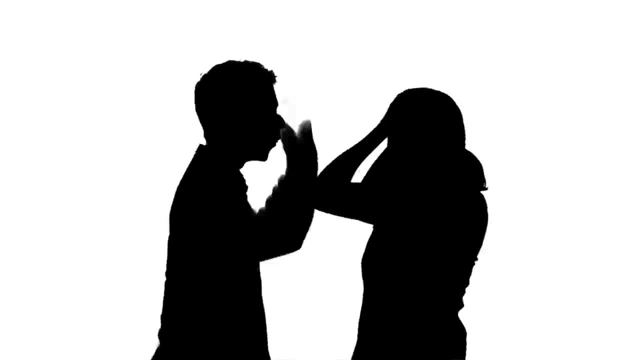 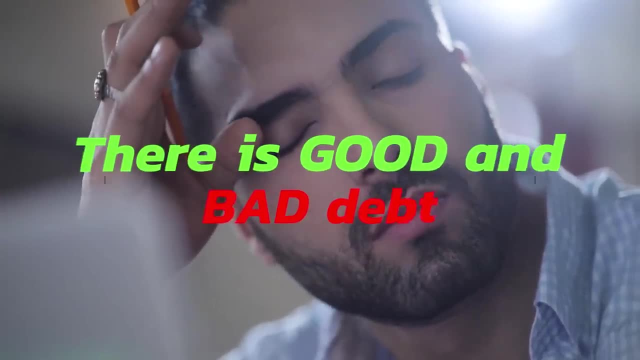 This one might be controversial, but the power of debt is underrated. All those that know how to use it will thrive, while those that are scared of it will miss a lot of opportunities. There is good and bad debt. Bad debt is anything that you know that you won't be able to pay off, For example, student loans. 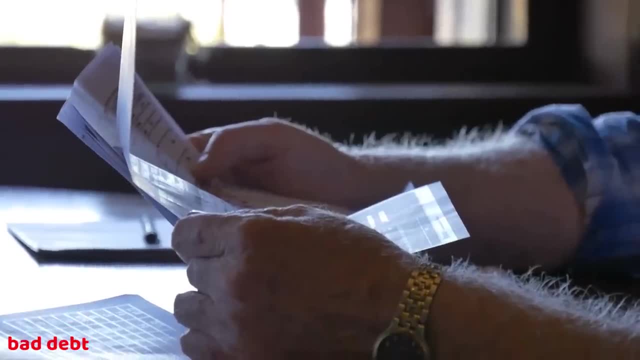 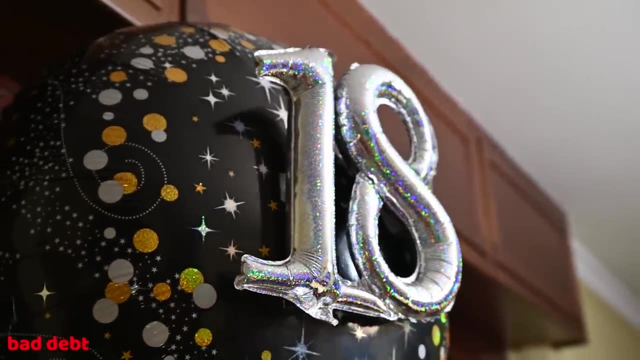 Bad debt is anything that you know that you won't be able to pay off, For example, student loans. This is extremely painful and it destroys the financial life of many people. We shouldn't ask 18-year-olds to make financial decisions of hundreds or thousands of dollars without considering the consequences. So be careful with that one and only get in debt if you know what you're doing. On the other hand, good debt is the type of debt that you're absolutely sure you'll pay off- or you have a plan to pay it off- and it will also make you money. 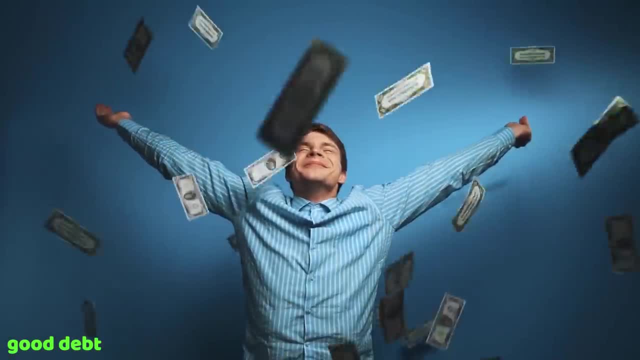 Getting in debt is a tool that you can use to get rich. For example, you might want to get a loan in order to start your business. For example, you might want to get a loan in order to start your business. For example, you might want to get a loan in order to start your business. 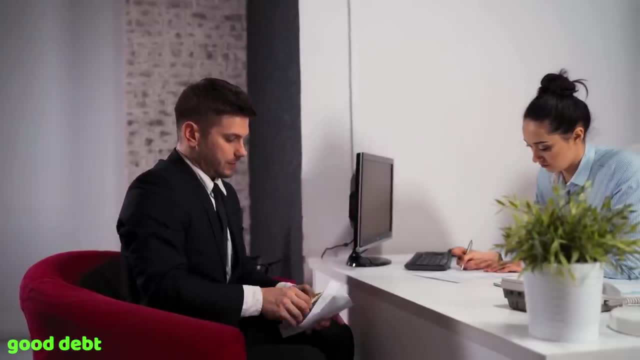 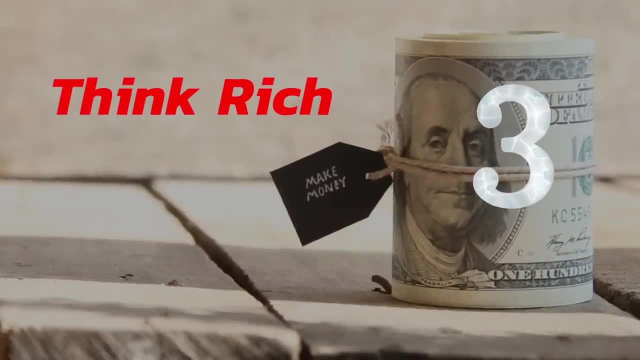 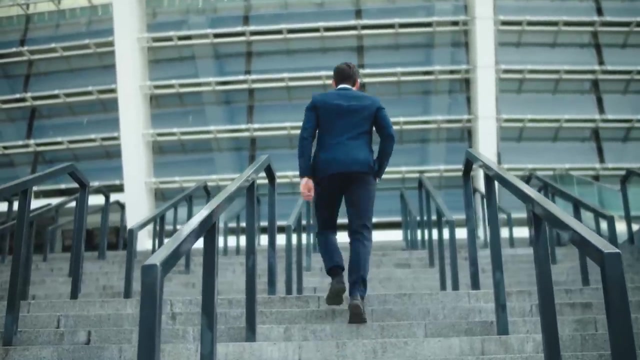 business. If all goes as planned, you will pay off your debt and will be free to expand your business, as long as you are always paying off your dues. Rule Number 3. Thank Rich. Thinking rich is seeing yourself rich and acting rich. Essentially, you are playing the role of a rich person, and this might include living. 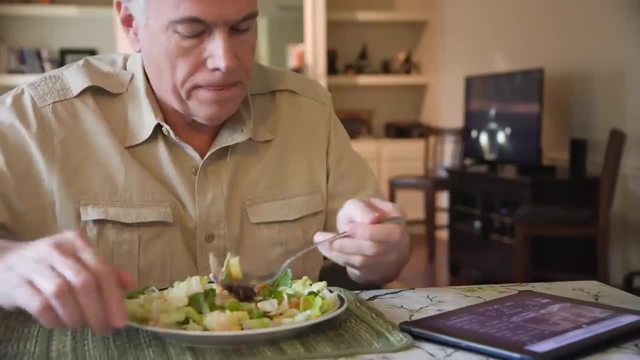 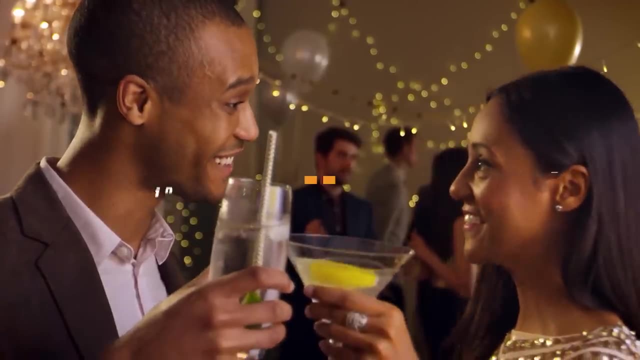 above your means. Living below your means is a defensive concept invented by financial gurus that, to the most part, is solid wisdom. I mean we shouldn't live way beyond what we can afford, because that is how people end up in serious financial trouble. 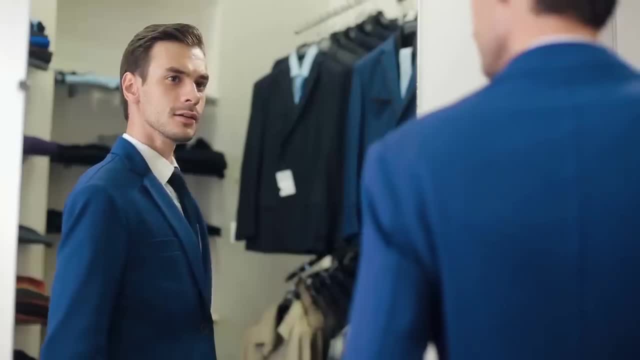 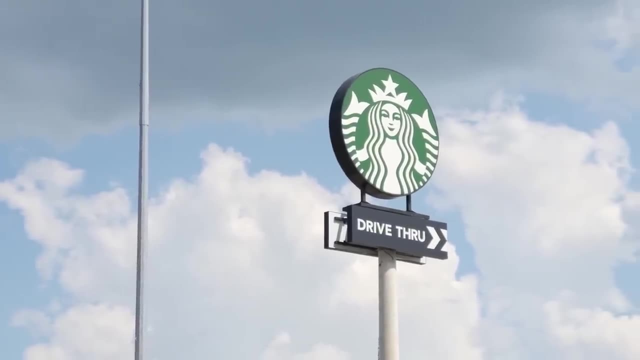 As long as you are disciplined and wise about what you are doing with your money, you have to also spend your money on things that give you confidence and make you feel good. Do you really think that depriving yourself of a couple of coffees at Starbucks will make? 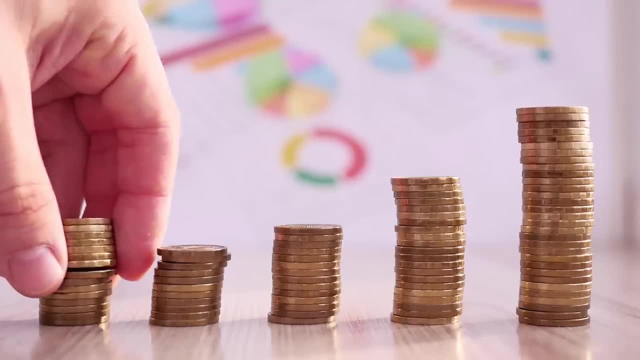 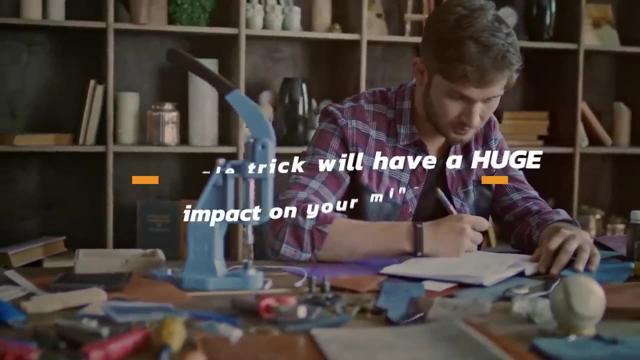 you a millionaire, Instead of living below your means and saving a penny here and a penny there, start gaining new skills that will make you money in order to support your desired lifestyle. This single trick will have a huge impact on your mindset. You will start seeing opportunities and places where you can make money.